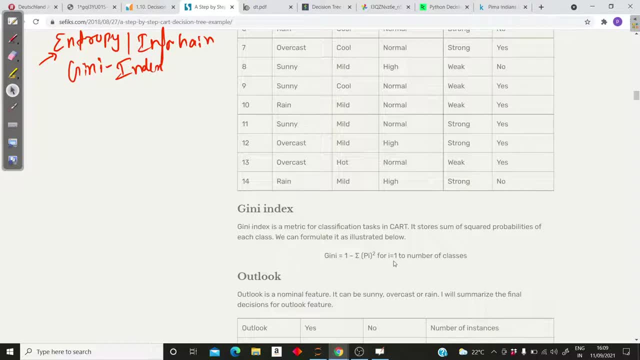 summation of probabilities squared of each classes. So I is 1 to number of classes, and this is nothing but the algorithm that is used in scikit-learn as well, and it is called CART. So what is this? CART is nothing but classification. 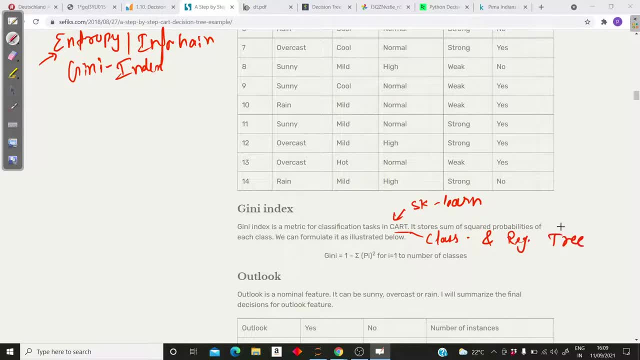 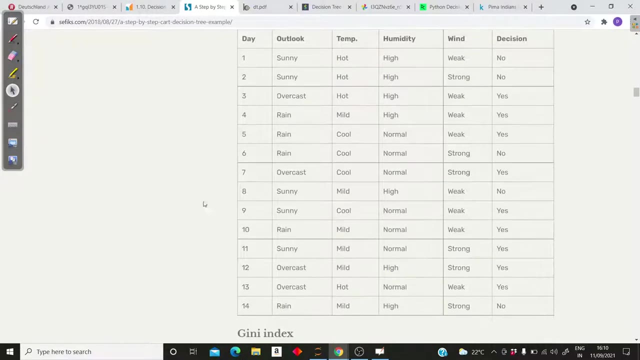 and regression. So we'll discuss this algorithm, that how it works, and basically scikit-learn uses this inside. So let's start step by step. So again, I'm taking the same data set. as you can see that this is the same data set: 14, our 14 number of rows, that is, data points. 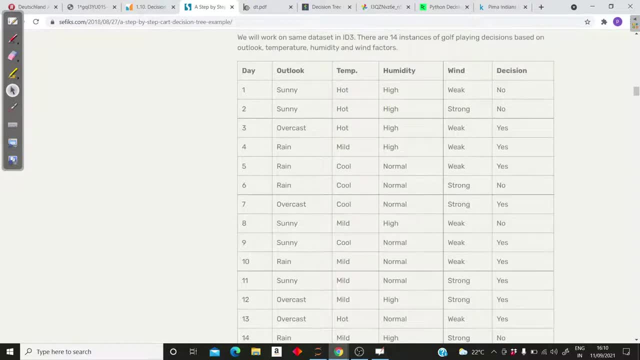 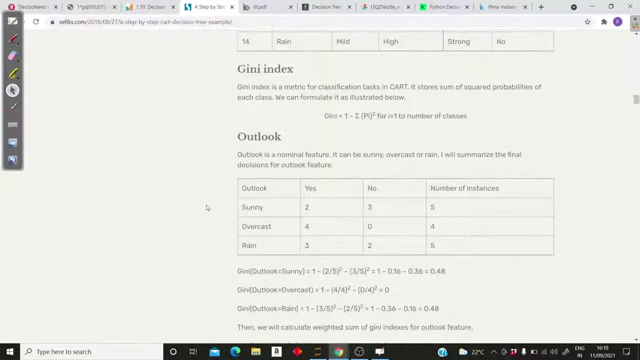 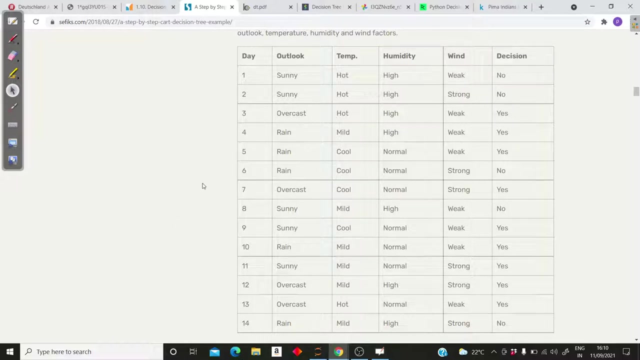 and we have to decide whether we'll play golf or not. here is just to play. decision is yes or no, based on certain conditions: The environment. so firstly, as I said, which one should be the root node. again, we will decide that which one should be the root node. So, in the last case, what we did was we used 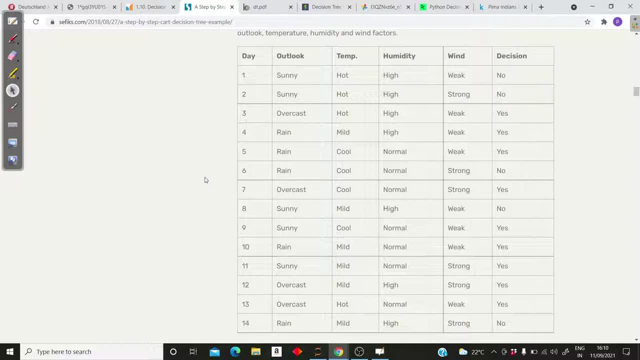 entropy we found the information gain and which was the highest gain that we utilized. Similarly, here, Gini is also also often written as Gini Impurity, So, as the name suggest, impurity should be as low as possible. The Hack I found, So here we'll see that. I hope I didn't count wrongly again This time. it Vou Irjl that we didn'taganastanise that 나가 смотрите Alright. So whatsoever: data��, Future giving of goods or urgently for certain conditions of the environment. 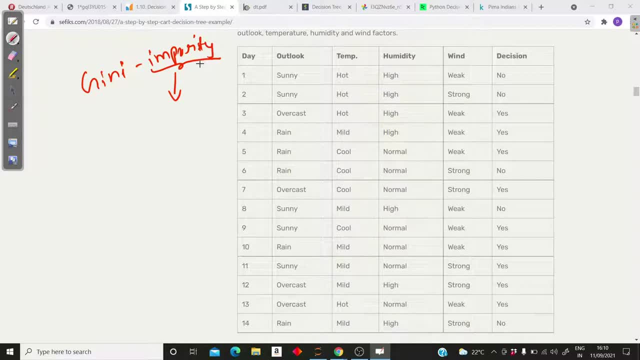 we will find a guinea impurity and based on this guinea impurity, when it is lowest, that we will select. we will count for outlook, temperature, humidity and wind, and which one is the lowest. we will decide that as our root node. so let's begin like that, just removing this, and let's 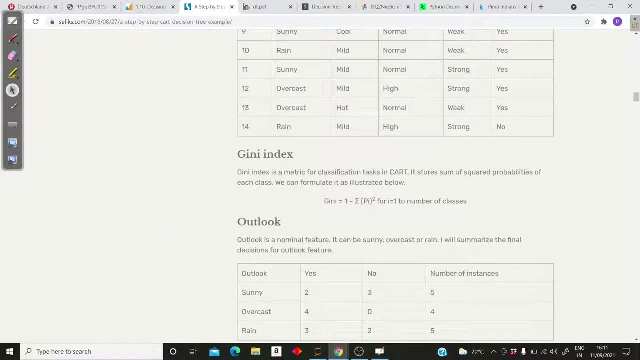 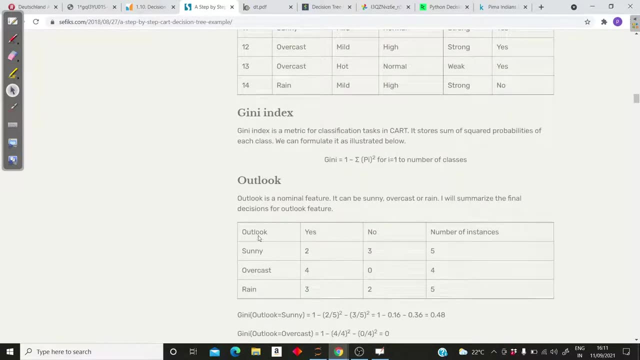 begin. so what will happen is that, firstly, we will calculate our outlook. so let's say in our outlook, what is happening is here. it's just like when outlook is there. what are the three possibilities of outlook? outlook can be sunny, overcast or rainy. so here we have. 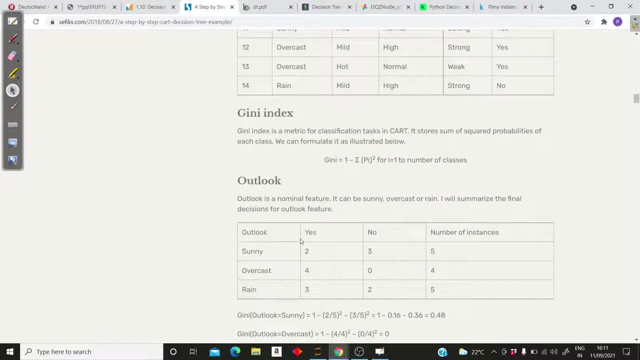 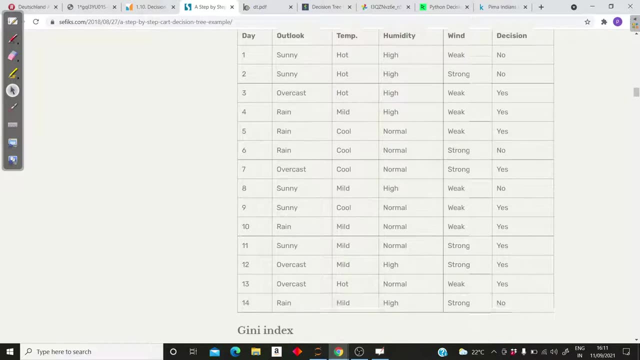 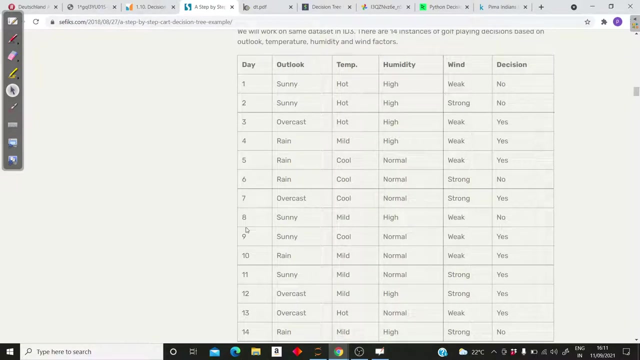 three possibilities. and when outlook is sunny, how many times we are playing? that is, how many times our outcome is yes, so the decision is yes. so, based on when outcome is sunny, two times, you will verify on the table that when outcome is sunny, you can see when it is yes. 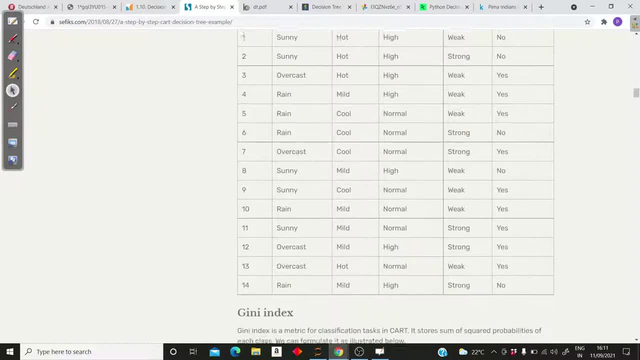 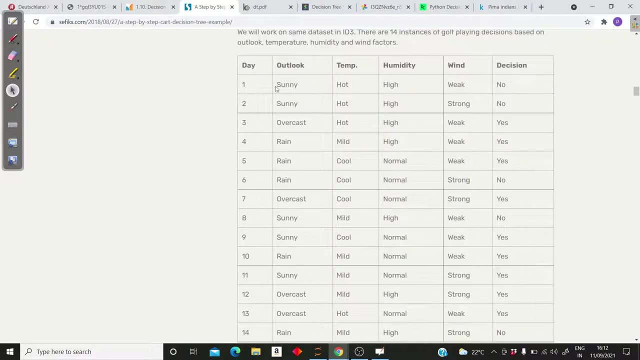 here 9 number: when outcome is sunny, we have yes, and here 11 number right and total. how many times we are having outcome as sunny: 5, 1, 2, 3, 4 and 5. so you can see that total we have 5 out. 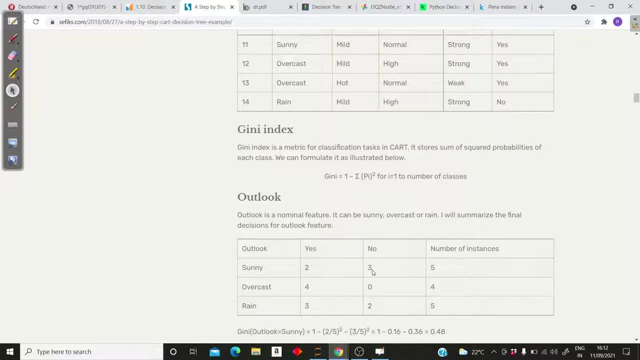 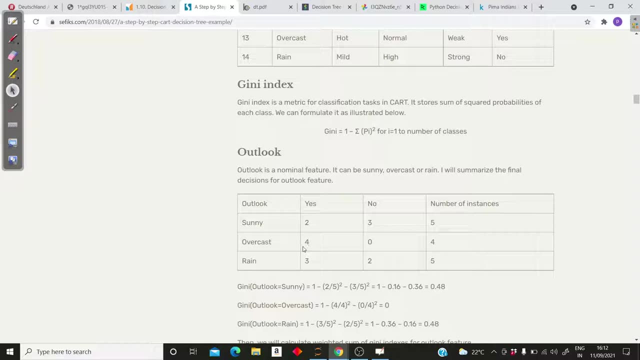 of this, twice we are having yes, and of course, then thrice we are having no. similarly, when outlook is overcast, we have this like bias, that when it's overcast it's always yes and 0 times no. so total 4 and all the times we will play, and similarly for rain: total instance. 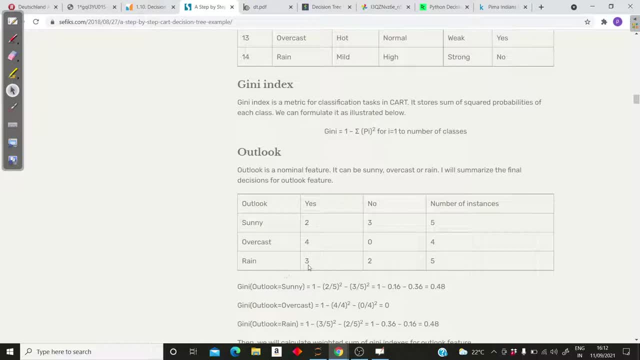 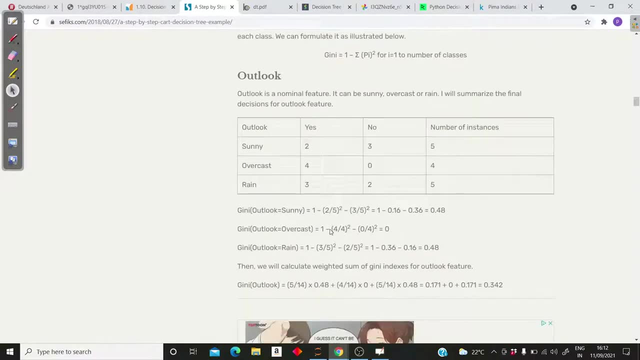 are 5. of course, this should be 14 in summation. so this are 5, out of which 3 times we are playing and 2 times we are not playing. so here you can see how we will find guinea. so, as I said, this is the formula. it is visible. so this is the formula that we have to just 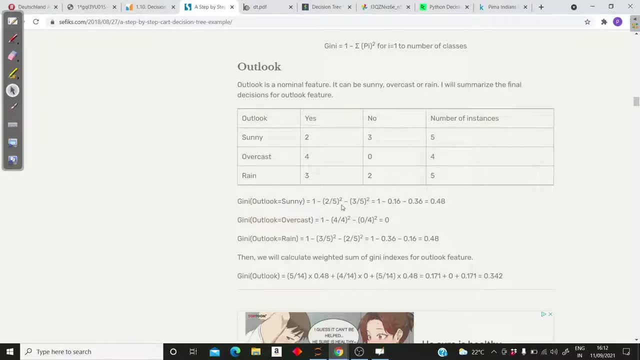 find the probabilities of each class. so guinea, when outlook is sunny. so what is happening each class, when it is yes and when it is no? here we have two classes, so two times out of five in total, right, we are having yes, so probability of yes will be two by five and similarly so it should be like if i'll take minus outside it. 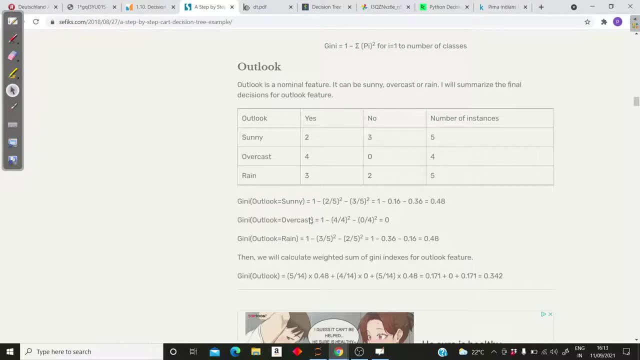 should be in the bracket and in between it is plus, because we have summation here right, but here minus is given to both the terms. that's why everything is in having minus. similarly, for no, we have three by five and squared. so if we will count this, we will get genie when outlook is sunny. 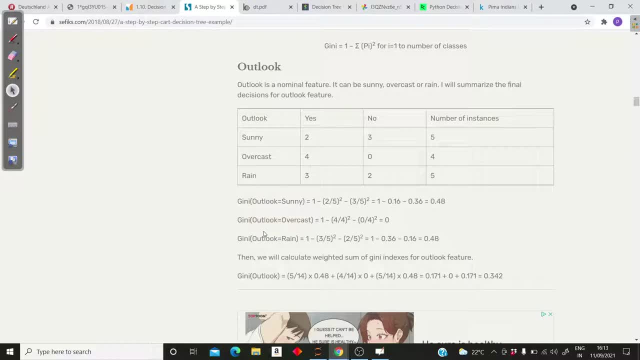 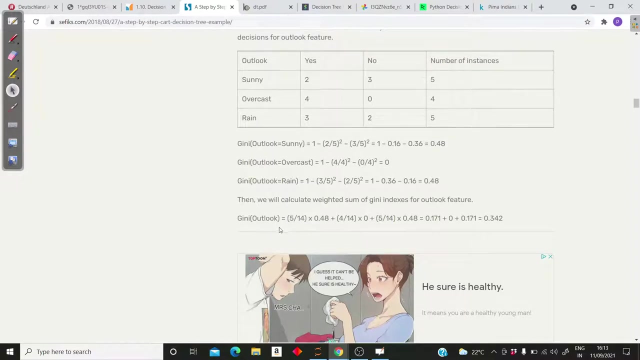 as 0.48, or i can say genie impurity. similarly for overcast, we'll get a zero, and similarly for rain, we'll get as 0.48. right, just by three, by five square and two by five square and one minus. now this is important, that this is the genie impurity when outlook is sunny, overcast and 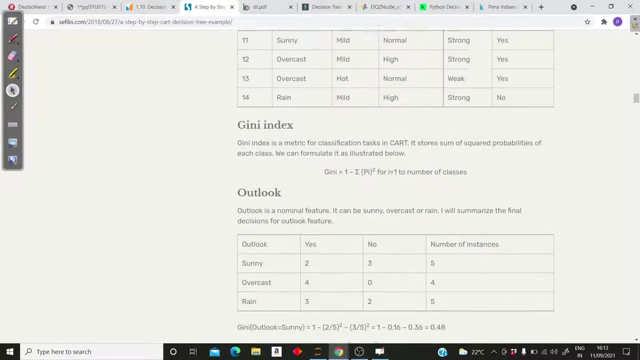 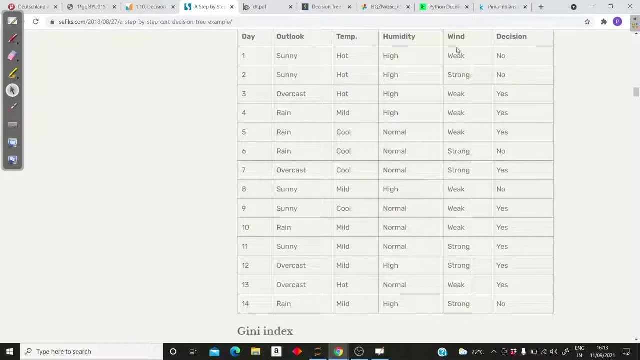 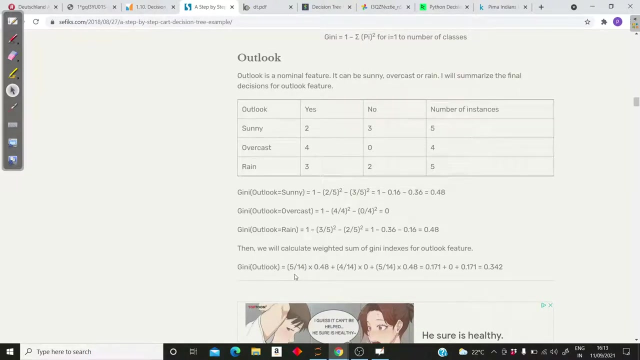 rainy. but actually we have to find for the node, because our node can be either of four terms right, or the outlook: temperature, humidity or wind. the root nodes can be any of this from this four. so at the end we have to find outlook genie impurity for the entire outlook node, yeah. so what can we do for that? for that, 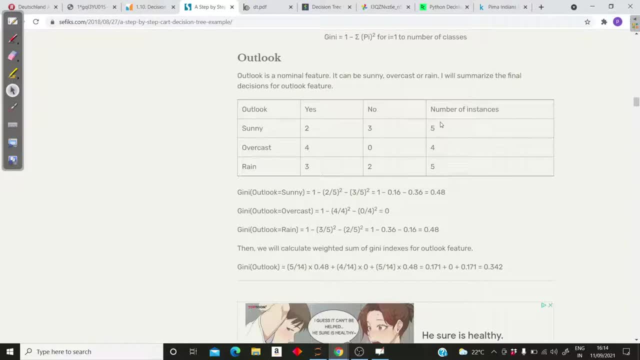 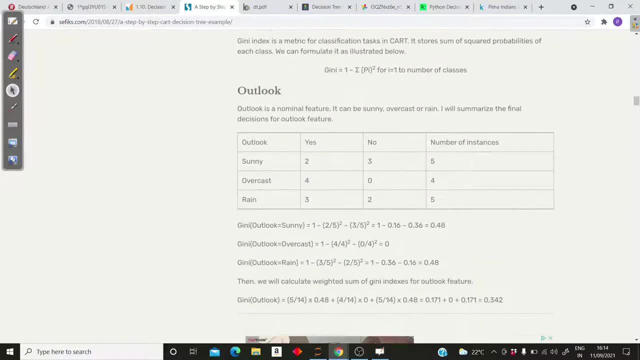 we'll just what we'll do. when outcome is: having sunny, we have total five and total we have 14. right, we have 14 instances. so what we'll do? we'll just wait. so, waited some. so when it is sunny, what is the genie? impurity. 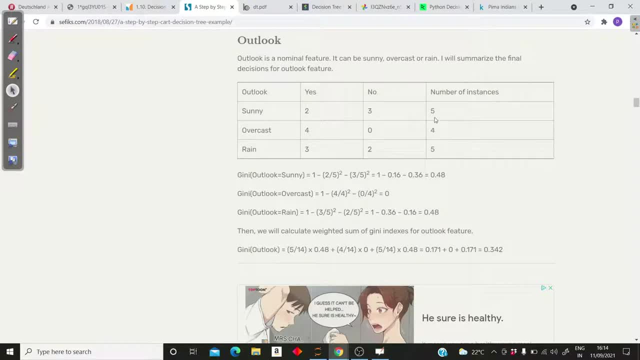 0.48. we'll just wait it by total number of instances. so it is five when it is sunny. total number of instances out of 14. so we'll just have 5 by 14 and we'll wait it. similarly, 4 by 14 and we'll wait. 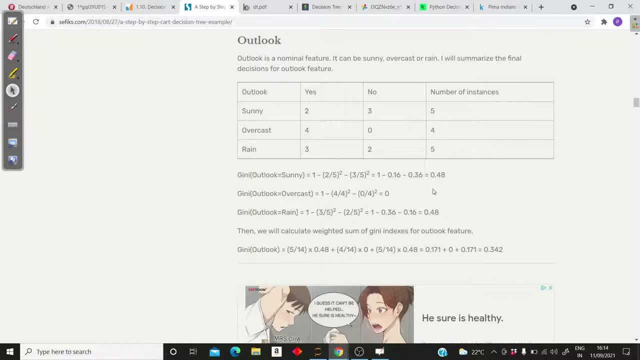 with zero, because for overcast is zero and for rainy we'll wait again with you can see 5 by 14 and 0.48 again, and what we'll get is this 0.348. so this that we got is the genie impurity for the. 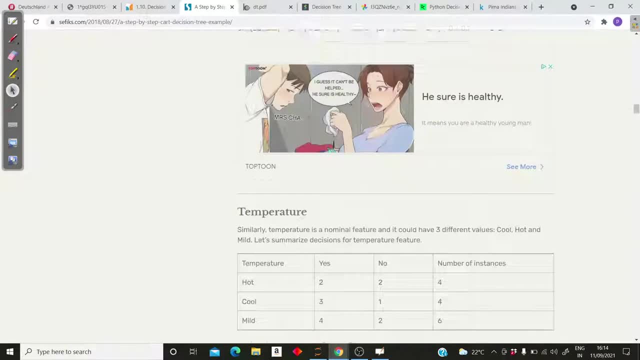 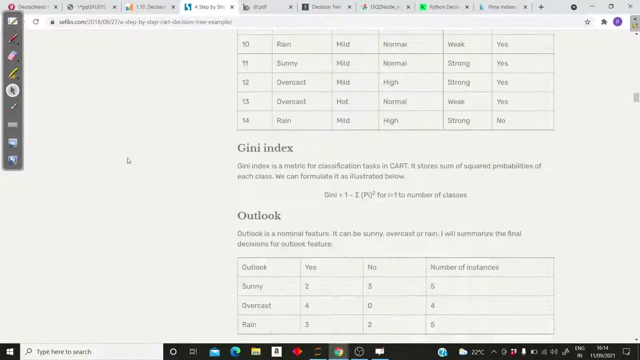 outlook node. so this is the genie impurity for the outlook node. so this is the genie impurity for the outlook node. then the same thing that we will follow for the temperature, because we have four things here you can see: outlook, temperature, humidity and wind. so the same thing will follow. 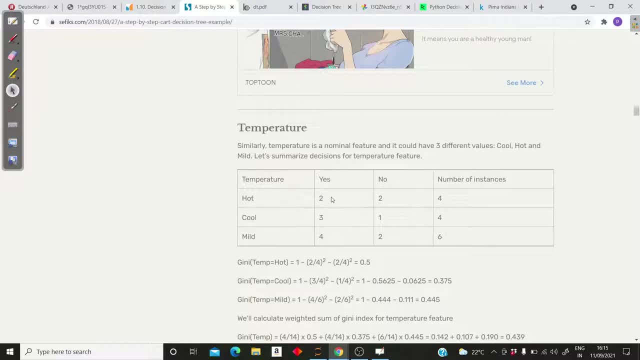 for temperature, that when it is hot, if you'll verify three times we sorry- two times we are having yes and two times we are having no. so total we have four times and two times we are having yes and two times no. similarly, when it is cool, total of instances are four. when it is. 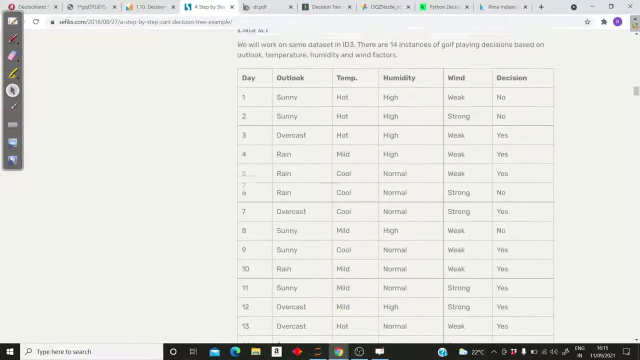 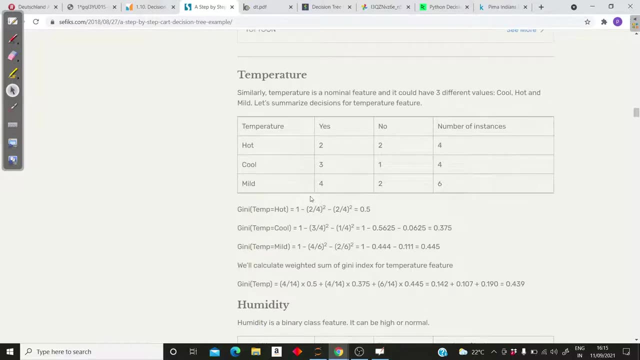 cool. you can just verify from the temperature. I am NOT going back, going back and forth every time, so same thing. we'll continue that how many times we're getting yes and no and based on that we'll just calculate gene impurity for each of the outcome of the temperature. that is hot, cool and 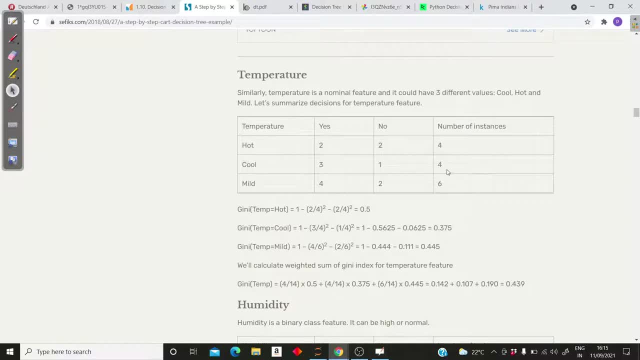 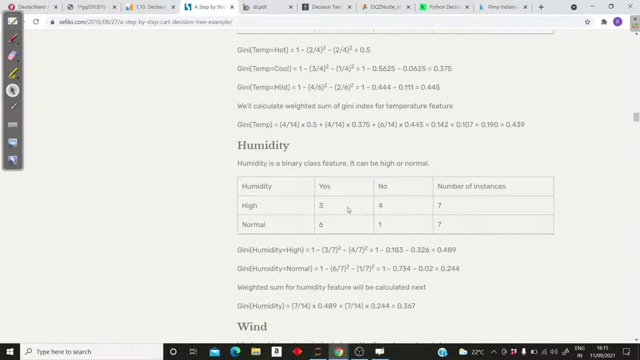 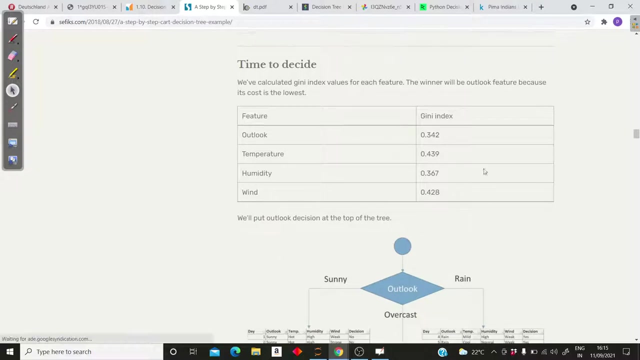 mild, and then again we'll wait it like 4 by 14, 4 by 14 and 6 by 14. so you can see, we will wait correspondingly and we'll get gene impurity like this. the same thing will continue for humidity as well, and the same thing for windy as well, and at the end, let us summarize that this is that what. 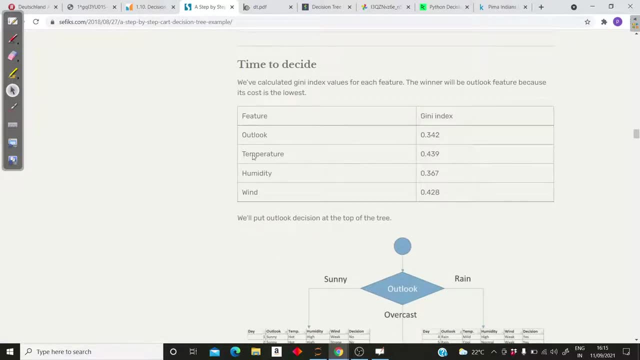 estreak whether this is done. the duty, then also, let us summarize that we are getting as compared to what we are getting. so it's time to decide now and, as I said, it's a impurity right. so we'll put the lowest one as our root node and you will see that the lowest from this is 0.342, and that's why 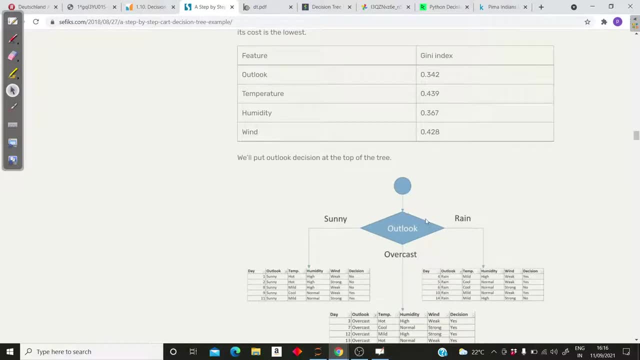 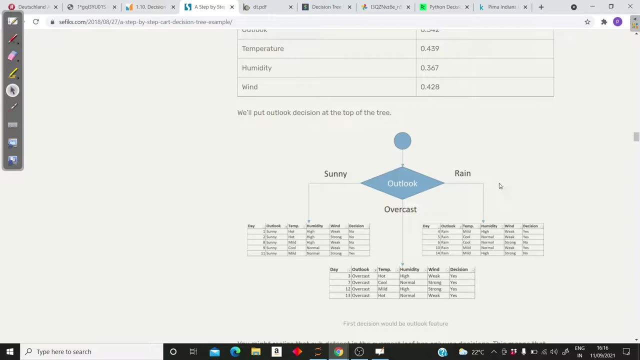 we'll use outlook as our root node. so our decision tree is being started now. we are building up our decision tree with the root node as our outlook now, as we know, that outlook has three things: sunny, overcast or rainy. so now we'll make our table. let me just zoom this a bit. 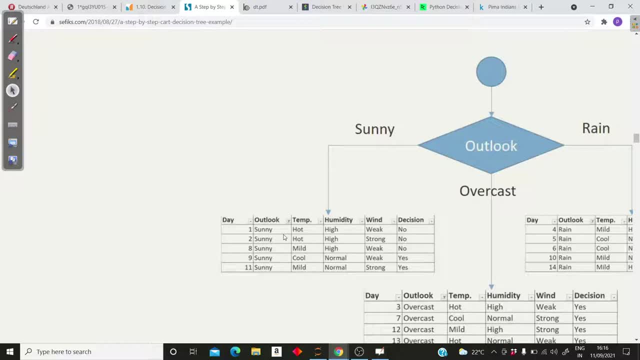 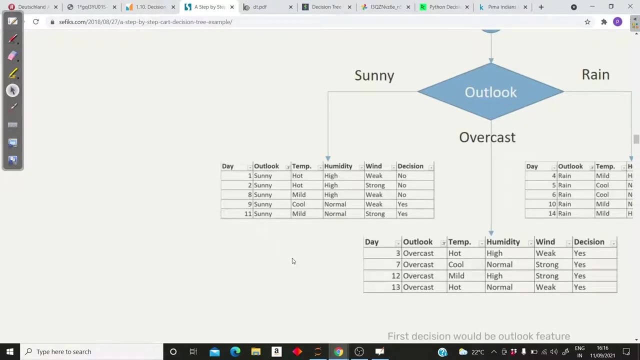 that how we'll make when it is sunny, we'll just, you can see- that when it is, we'll just take all the outcome which is sunny, because now we are just focusing on when outlook is sunny, then what is the table we are left will? it will be obviously the subset of it. similarly for overcast. 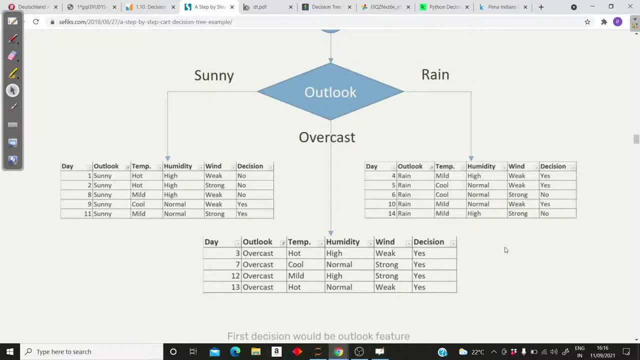 we'll do this and similarly for rainy, we'll do this right that when our outlook is rainy, what is happening now, what we have to do? we have to decide what to choose here, right after outlook is sunny, what to choose from temperature, humidity and windy. sometimes we can. 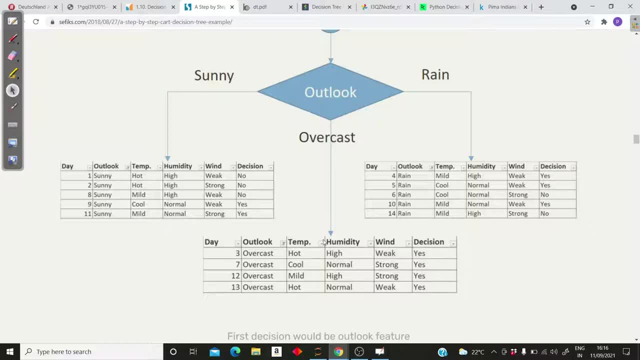 just directly decide. because here you can see, every time decision is yes, irrespective when outlook is overcast, you can see that irrespective of temperature, humidity and windy value, the decision is yes. so for this thing we don't have to decide, we'll just say that this is our leaf. 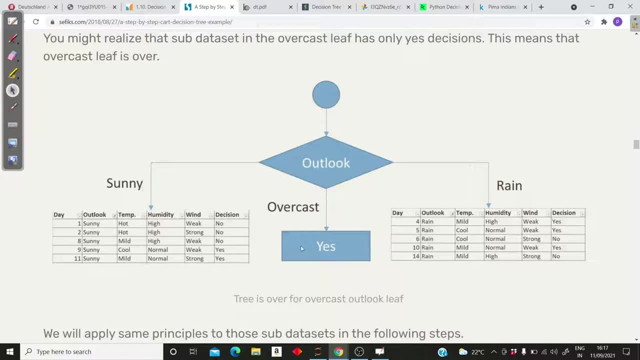 node now and we'll say: just say yes. so you can see that here it's always yes. so when it's overcast, we'll always play, irrespective of anything. whether it's temperature is cool, mild, we don't care. humidity is there, windy is there, we don't care. but when it's overcast, we will play. 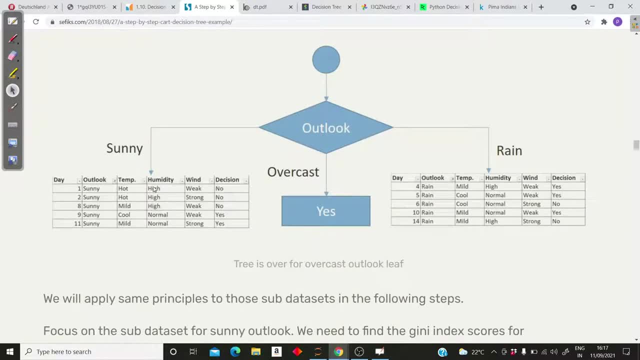 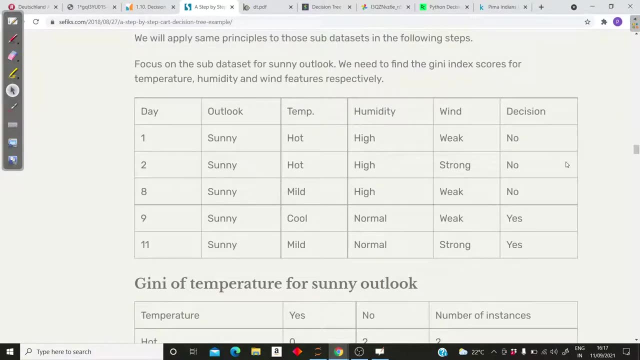 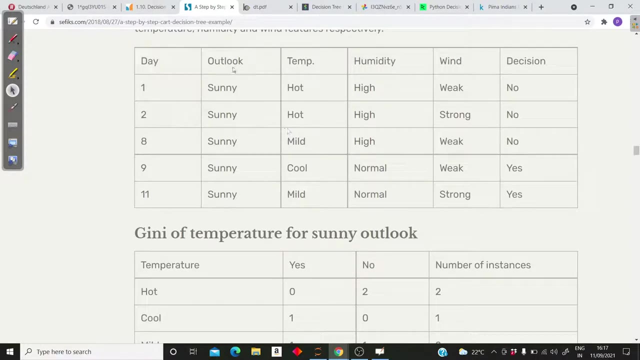 now the question is: we have to decide for here sunny and for rainy. so let's go step by step. so again, what we'll do is that when our outlook is sunny, we'll check for temperature, because we have to decide for temperature, humidity and wind. so let's get rid of this outlook now, because we 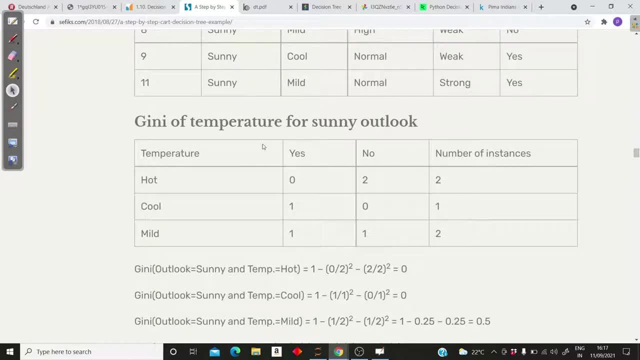 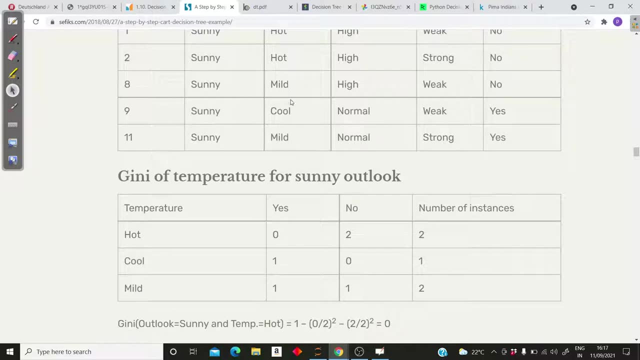 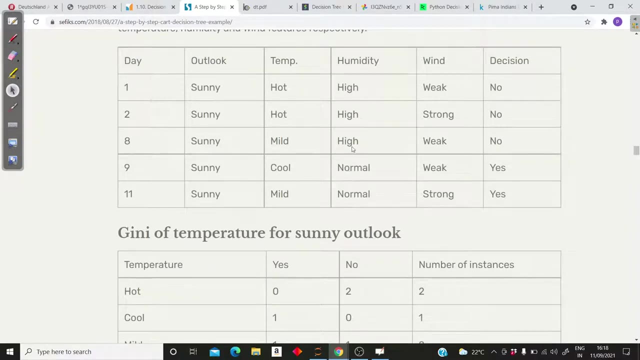 know it's sunny now, when outlook is sunny, we'll check for temperature. so we'll find the unimpurity for temperature. so again, how many possibilities are there- hot, cool and mild- so for temperature- again hot, cool and mild- and how many times it is happening, so you can see hot is happening twice. 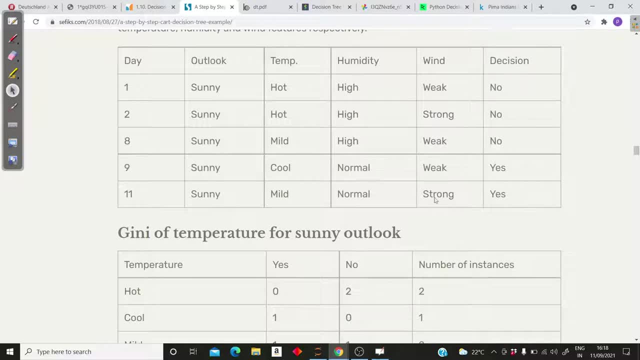 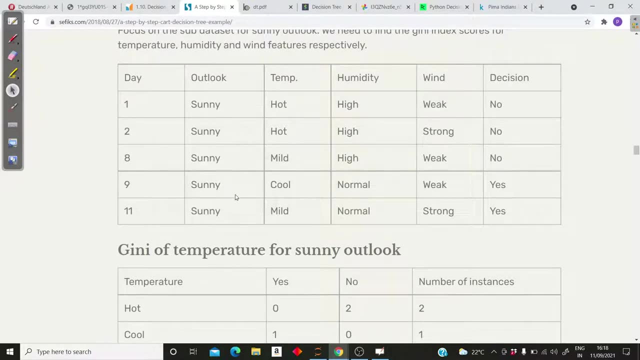 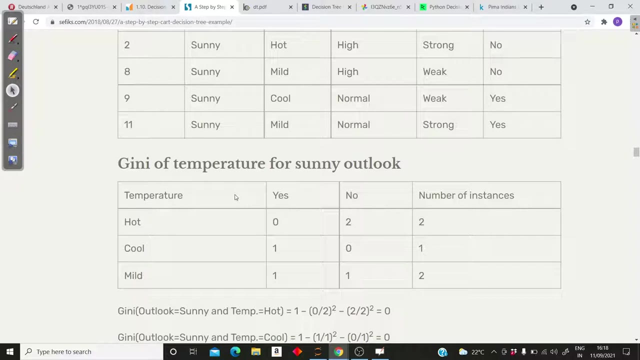 here and in both the times we are having no. so we'll construct the table based on this. now, yeah, that we get, when we have conditioned that our outlook is always sunny because we are calculating that node. we fixed our root node, that outlook. then sunny, it's fixed. so we are calculating now the parent, child node of this parent node. so 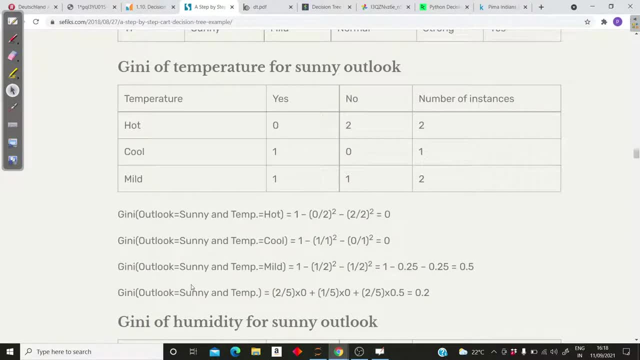 again, we will calculate the same thing that when outlook is sunny, of course, for all the four cases, but when temperature is hot, cool and mild, and then we'll calculate all the Gini impurities and then we'll take the weighted sum again that here total instance are five. so we'll wait this by two, by five. this is: 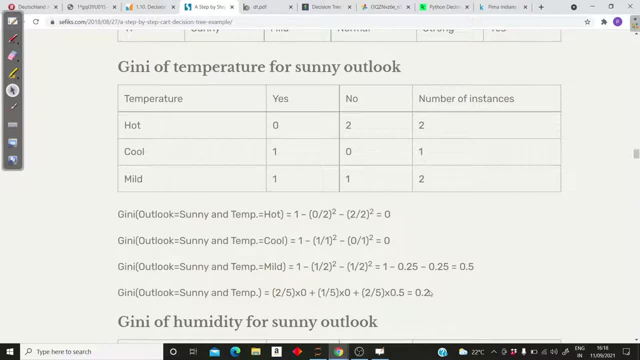 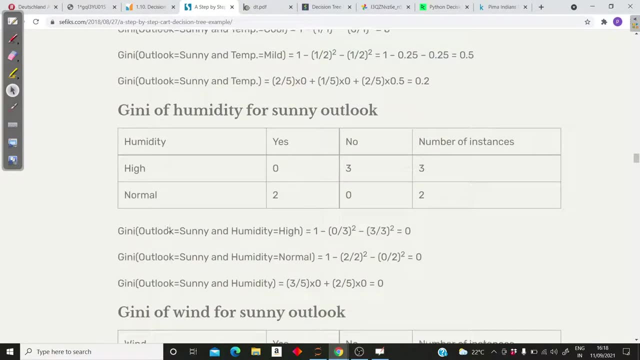 one by five and this is again two by five. so we are doing the same thing again and we are getting 0.2. the same thing will continue for humidity and for windy, provided when outlook is sunny, and at the end we'll have a time to decide. 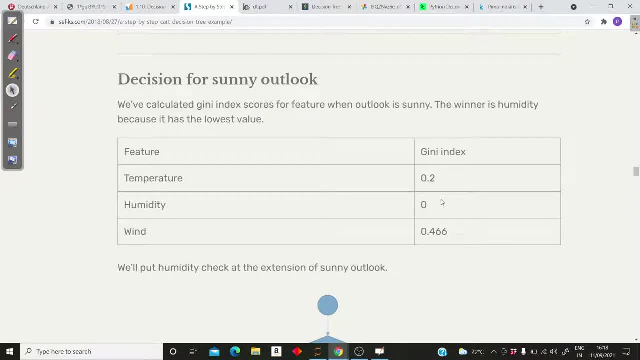 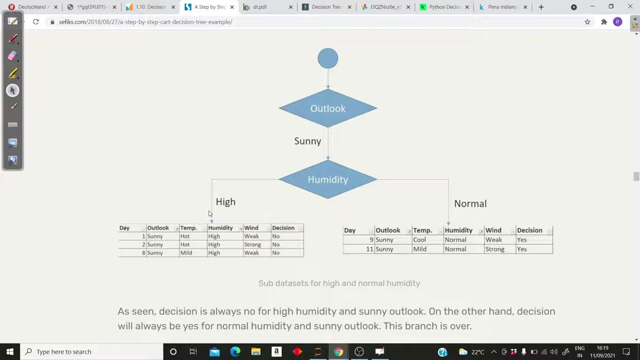 that what? what will have? decision for sunny outlook that this is what we are going to have: zero point two, zero and zero point four, six, six. so of course will decide for the lowest one and lowest is zero. so we'll say that here humidity will work. yeah, so here. 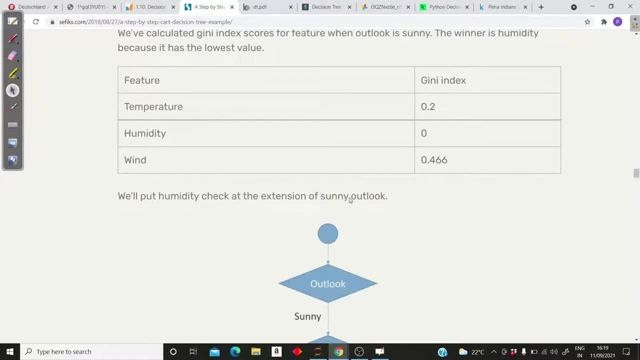 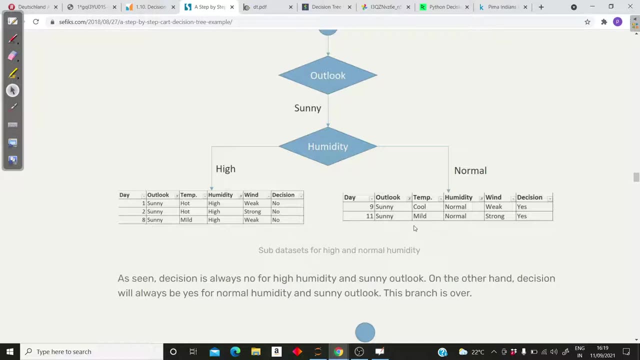 humidity should be, so we'll put humidity check at the extension of sunny outlook. similarly, we'll proceed for this. that so, as we as seen, decision is always no for high humidity and sunny outlook. on the other end, the decision will always be yes for normal humidity and 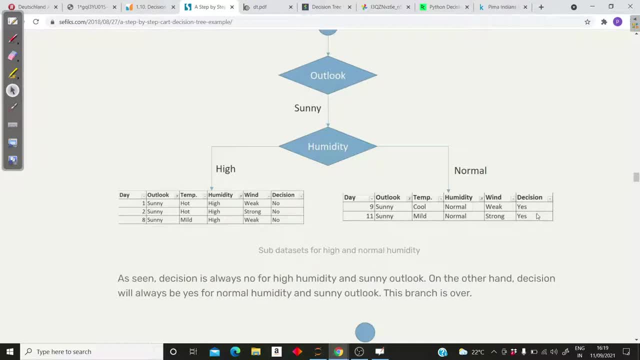 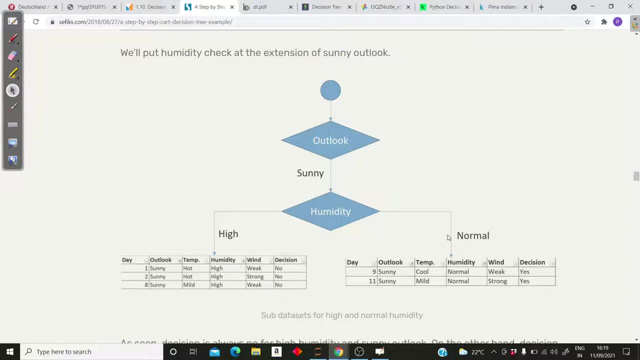 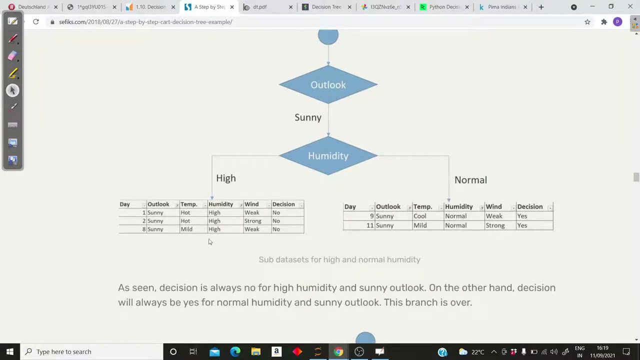 sunny, outlook, correct. so here you can see for normal humidity. so this is just: we are focusing on outlook sunny, then it is high and it is normal, correct? so we are first putting humidity and then humidity has just two values: high or normal. so you can see that for high. 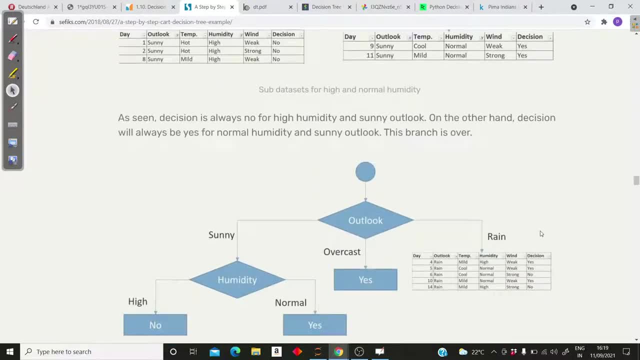 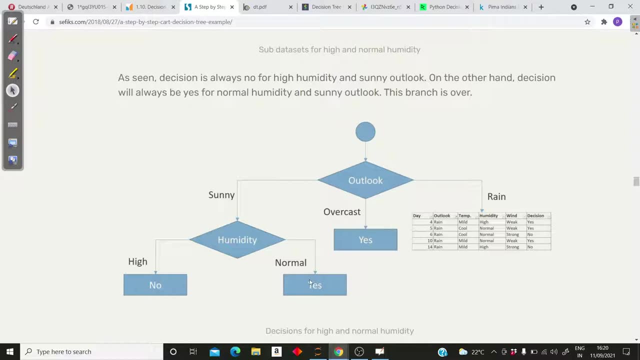 we are getting always no decision and for normal we are getting always yes decision. so we can just directly put our leaf node here. that humidity high, then no normal, then yes. now time to decide for this. we are done with sunny and overcast because we had leaf node now. 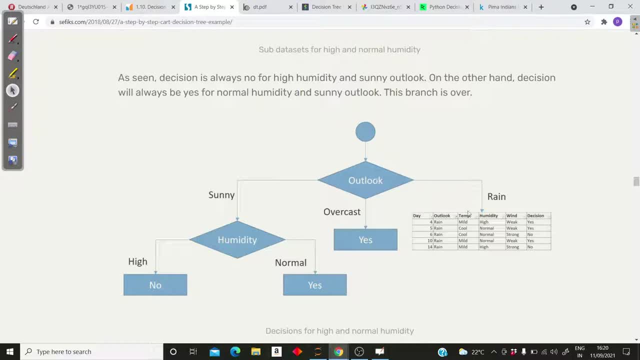 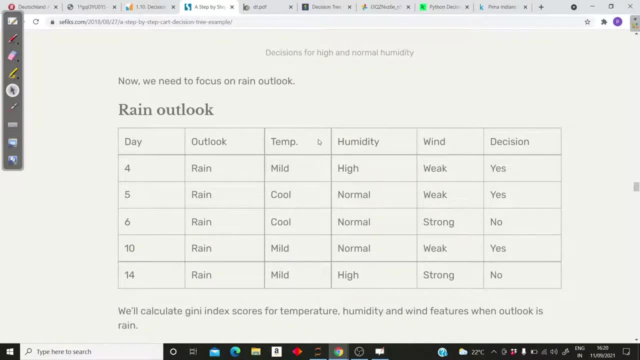 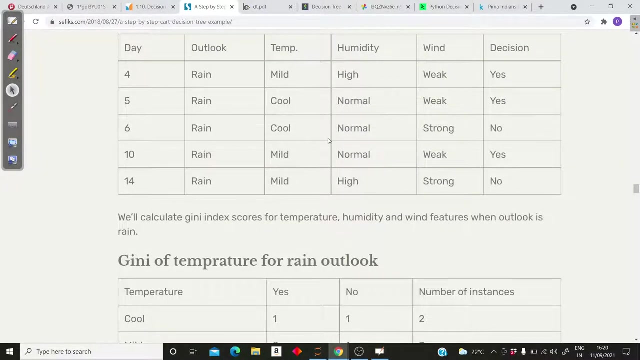 after leaf node, our decision: tree can't grow anymore, then just decide for rainy and we'll proceed with the same thing, that we'll check when outlook is rainy, whether we'll have temperature, humidity or windy. so we'll check again the same thing from this table. as i said, we have to build. 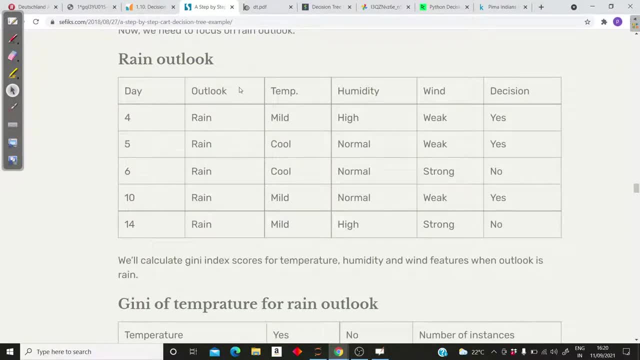 this table based on this subset of the table now, because we condition that our outlook will always be rainy, so we have to build this table based on this subset of the table now, because we condition that our outlook will always be rainy, so we have to build this table based on this subset of the table. 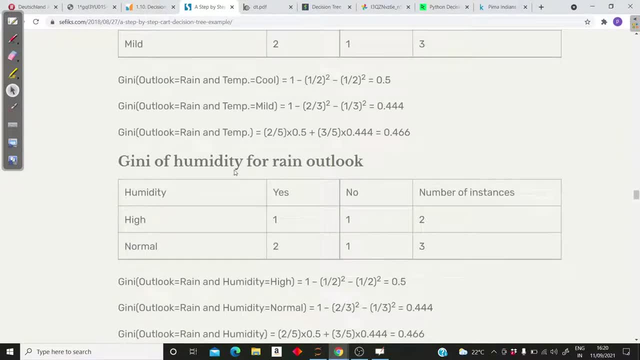 just consider those instances where outlook is rainy, then we'll proceed. the same thing again. we just consider those instances where outlook is rainy, then we'll proceed. the same thing again. we are checking for all the three and then we are checking the decision and you can see we are. 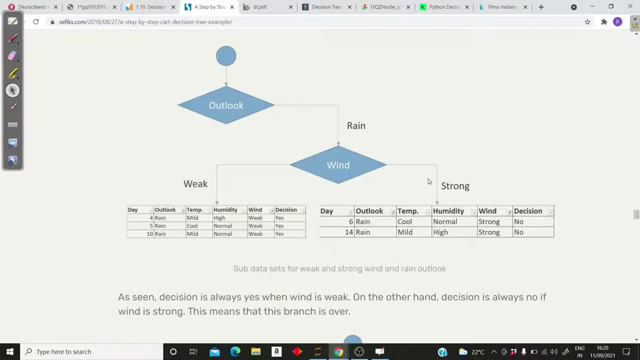 are checking for all the three and then we are checking the decision and you can see we are getting lowest as windy, so we'll put windy here and then we'll see when, whether wind is weak or getting lowest as windy. so we'll put windy here and then we'll see when, whether wind is weak or 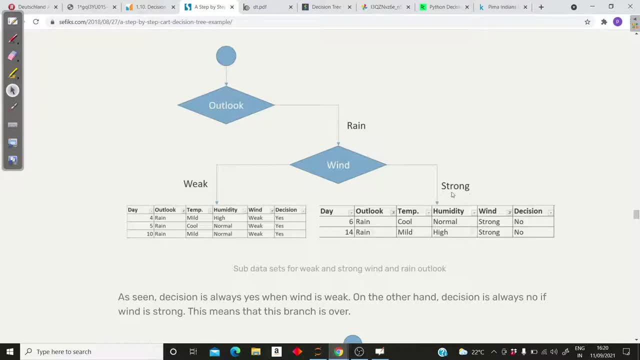 strong, so for weak we are getting always yes, and of course when there is strong wind we can't play strong. so for weak we are getting always yes, and of course when there is strong wind we can't play. so again we are having our leaf node and if i'll proceed or if i'll compare, sorry. 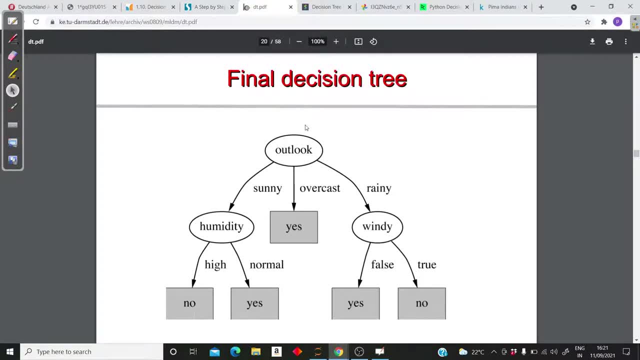 so again we are having our leaf node and if i'll proceed or if i'll compare- sorry with the last time, so in the last lecture, four point to what i showed was we made this decision tree based on entropy or the information gain, and if you will compare you will get all the same. 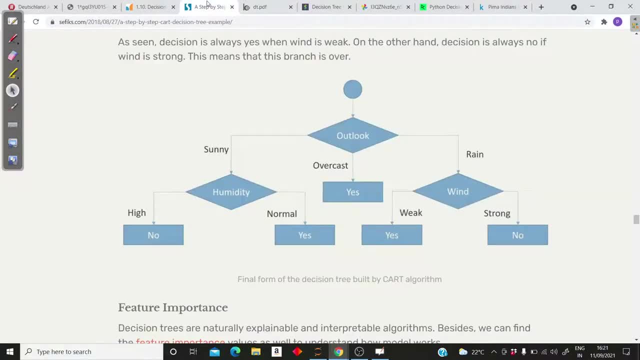 thing, yeah, that you can see the. both the trees are the same. so whether you will use genie impurity or information gain or entropy, so information gain or entropy based approach, or you used genie impurity- both give the same result or same kind of decision tree, but this is computationally less expensive as compared. 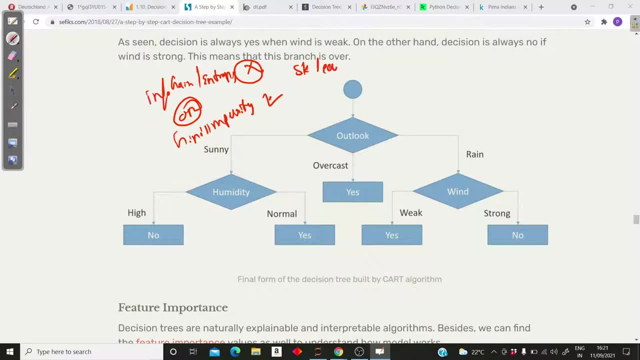 to this and that's why scikit-learn avoids this and scikit-learn uses this that i just explained. this is called cart algorithm, correct, and there are many important things that i can show you for decision tree, that for decision tree, there is a feature important that will 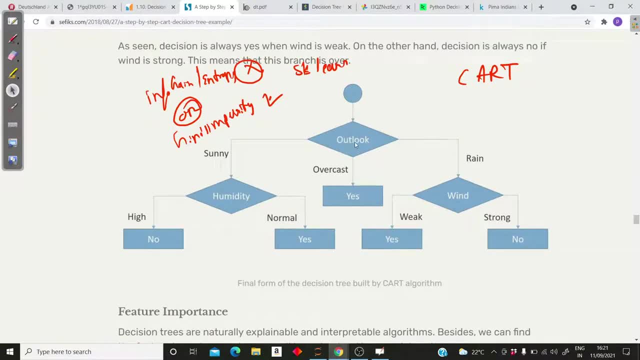 get the importance of the feature right, because we can see everything here, that what is happening in here, and that's why i said that it is a white box algorithm like other algorithms, like neural network, we can't say which neuron is firing and all we can't see inside. that's. 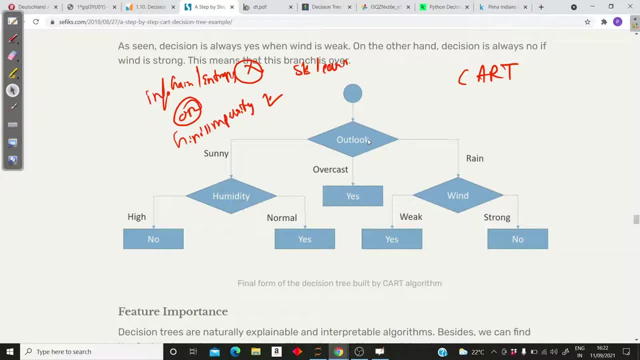 a black box for us. we can just see the output that it is giving, but we can't say that this is happening because of this neuron is firing, or we can't say anything, but here we can see everything because it's- it's like a flow chart. yeah, that, whether it's condition satisfied. 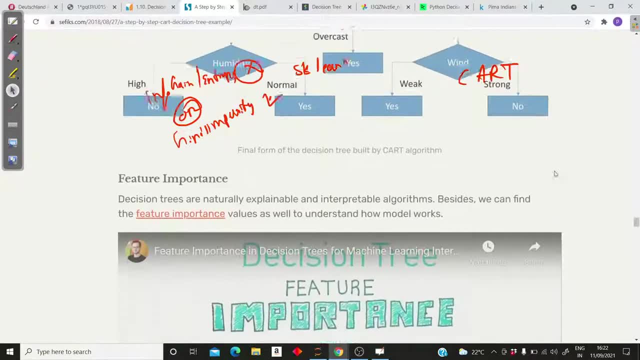 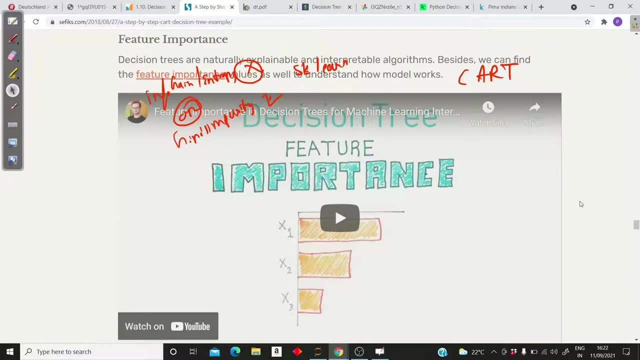 we'll do this, that, so it's just like we can see everything what is happening, and that's why we can say it's it's having feature importance. so which feature is important and which feature are important, we can consider them, and which are not, we can neglect them. we'll see all. 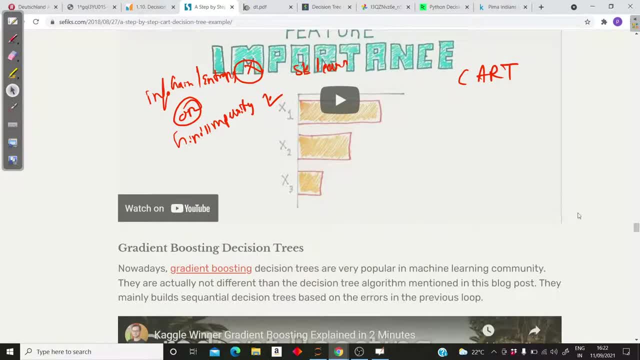 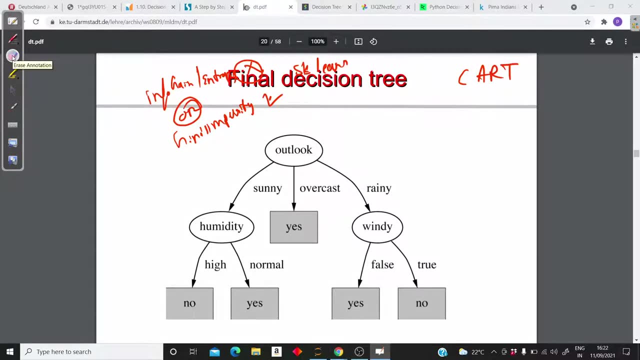 this thing when we are considering our random forest lecture. so, as of now, what i can say is that at both the approaches are giving the same decision tree, as you can see. so it's just like your choice that, whether you choose this one or that one. so let me just quickly. 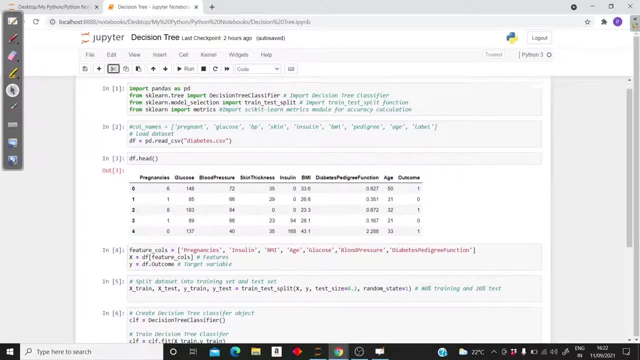 go to the core part now that. so this is the code that we are going to see for decision tree. so here i'm just importing little ideas with our fossil field talking, and right now the driving force is changing here. so two remaining traces define what's happening here. 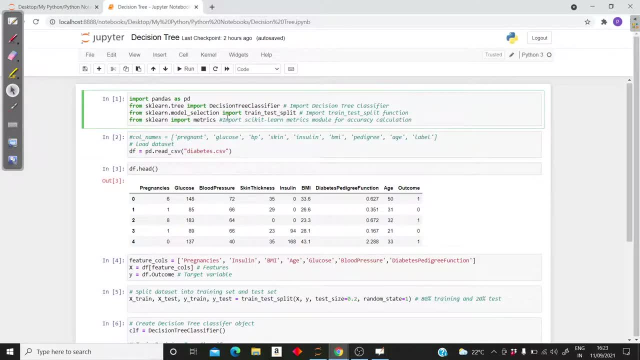 what is happening where, what is happening here, fafz, and why, as you can see, this which go longest: ancestry libraries, and I just have all the comments. so this is for pandas, this is for decision tree classifier, this is for training and test, data splitting and these are some matrices like we'll use accuracy here. so let me first show you. 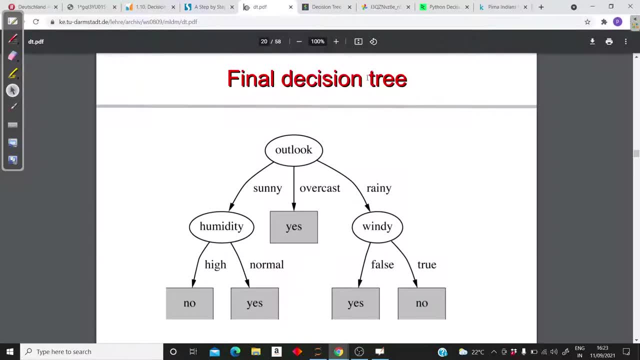 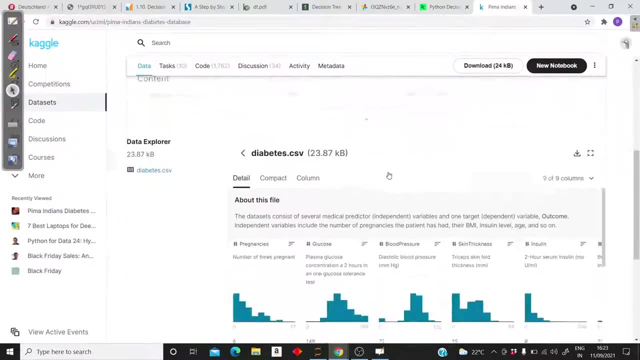 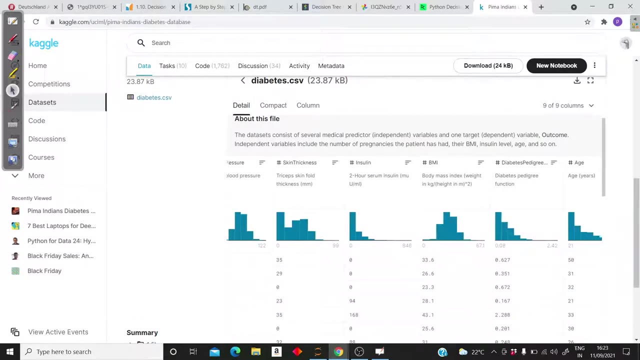 the data set that we are using. so, okay, here is the data set, so it will take time to load, I think yeah. so it's a diabetes data set and you can see that there are many columns like pregnancies, glucose, blood pressure, skin thickness and everything you can. you can see everything here. that. what is BMI? some? 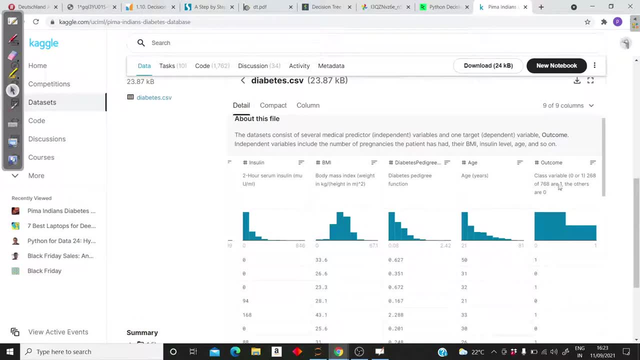 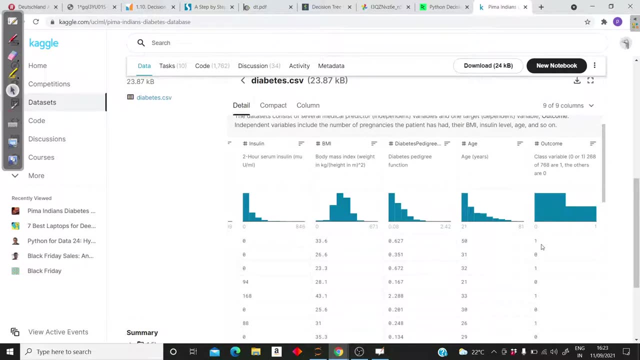 these are some biological terms, that age and all. so we are interested in outcome. yes, that based on all these values, can we say that the patient is having diabetes or not. so one means he has diabetes and zero means no. so we have to create one classification algorithm based on decision tree. that, whether our 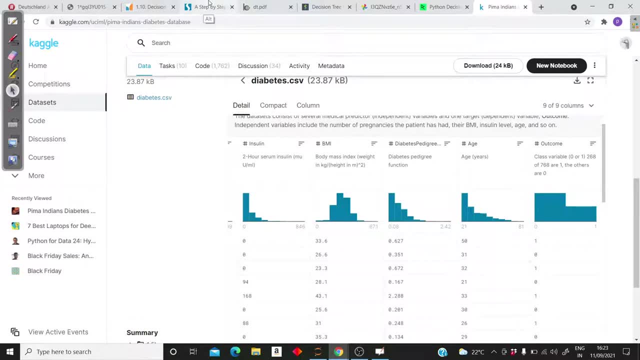 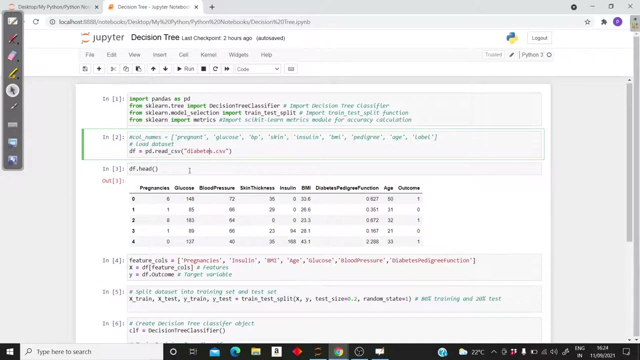 patient is having diabetes or not, so will see the same here that I just imported this data set just so you can. what you can do is you can just download it from here and then put the zip file in your working directory where this python notebook is and you can just read it. so you can see that there are many columns here. 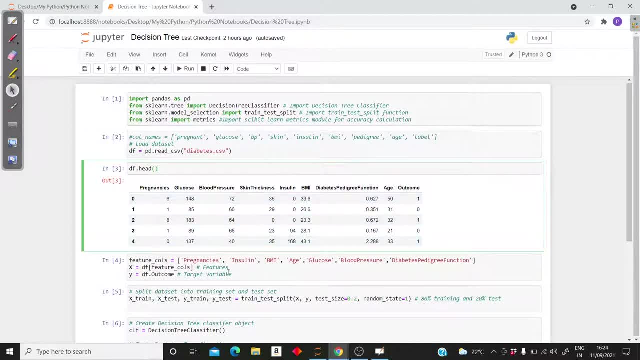 so what I'm doing is because what we want is that our input, that is, x, should be just this: columns up to age, right? this, all are the features, but outcome is what we have to predict, so we have to remove it. so X should be our training data, and why so? why should be your outcome, right? so 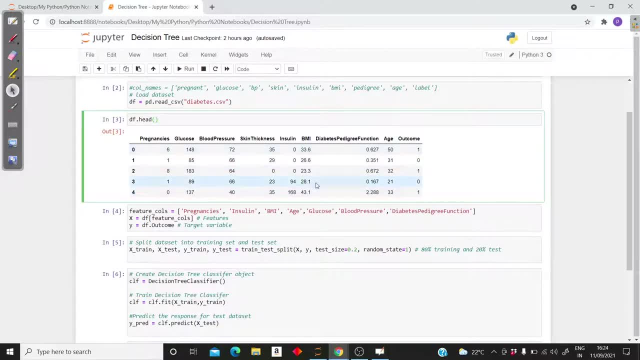 X should be our features, not like training data is totally, and training data will split it train into train and test. sorry, I can't say that it's a training data, but I can say X is all the feature values and Y is the outcome based on that feature. so here I just wrote it that X is all the features. 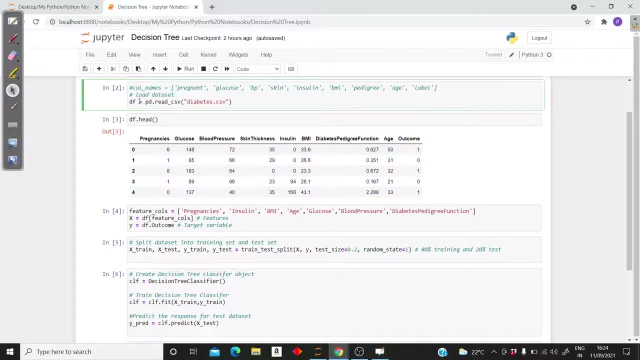 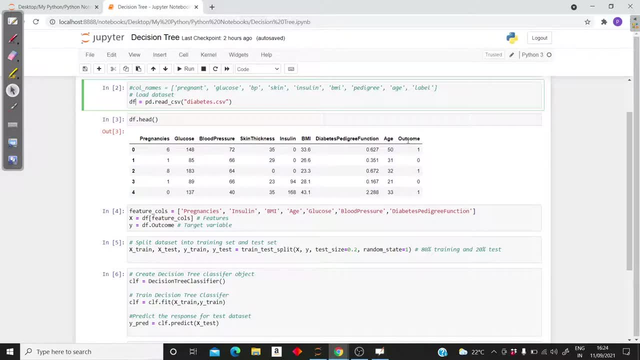 and I'm just giving feature column, so I just give all the names from here: pregnancies, glucose, whatever name was there in the data set. and I am now after having X&Y. I am just splitting the data into training and test, so here is the part where I am. 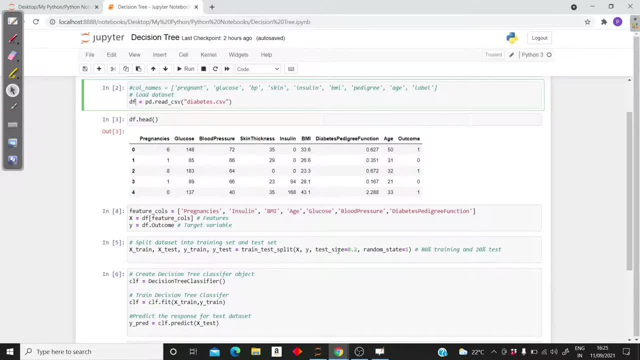 splitting it and you can see I have 0.2. so it's like I have 80% of training data. so I'm the total data I just having. I am just showing first 5 entries using head, but you can see how many total entries are there. I can just show you here as well that in total you 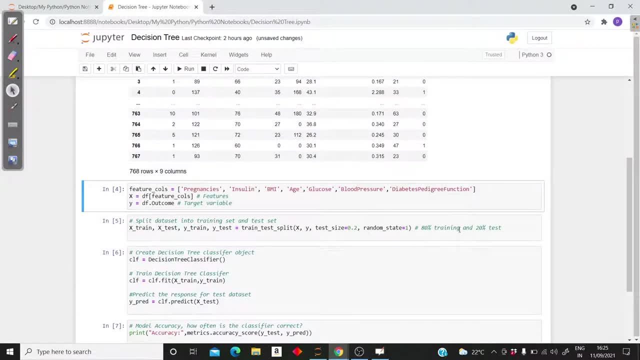 can see, there are 768 rows. so based on that, we are dividing 80 percent into training set and 20 percent randomly. you can change random state here and this also can give you more accuracy or less accuracy. this is hyper parameter, you can modify it, so it's like random set is just like how it's. 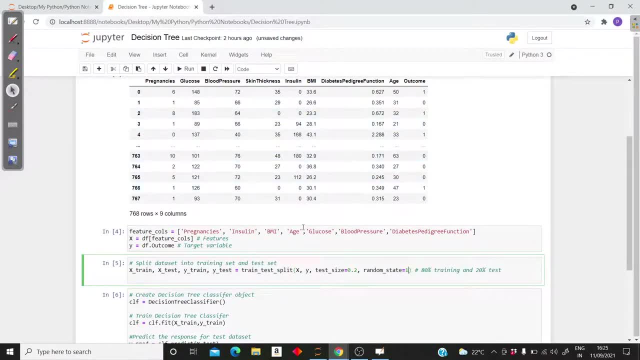 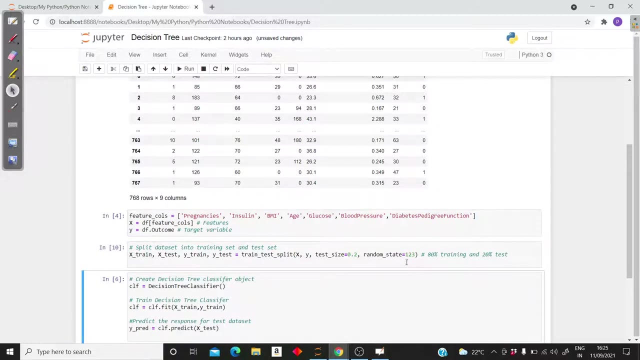 gonna choose 80 percent of it. so one way is that it's not like one means that it will choose one, then second, then one after the other, like one then three and five. it's not like that, it's the random thing. so if you'll put one, two, three, it will also work, doesn't matter. so based on the random state. 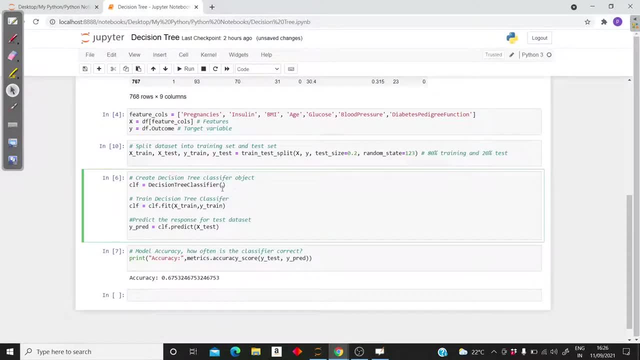 it will choose this. then here what we are doing is we are just invoking our decisionary classifier and storing it in our clf variable. then this is the training. so we are just training clffit, x train and y train. so now our clf is a train decision tree and then we are testing our train. 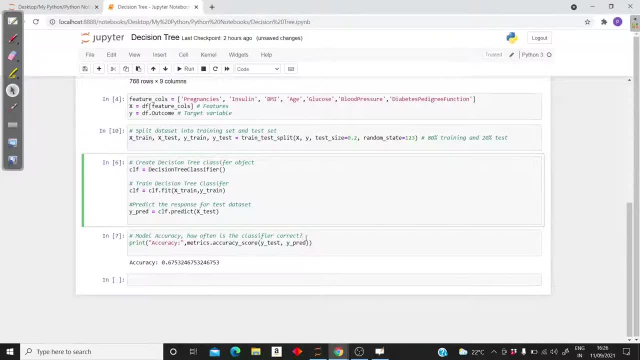 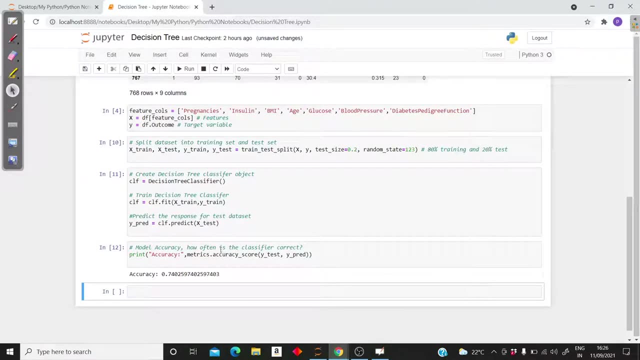 decision tree on our x test, which is our unseen data, and then we are predicting the accuracy and you can see we are getting 67. now i change the random state. let me just try again that whether i'm getting anything else. yeah, so i'm getting 74 now, so you can modify this thing using the random state. so 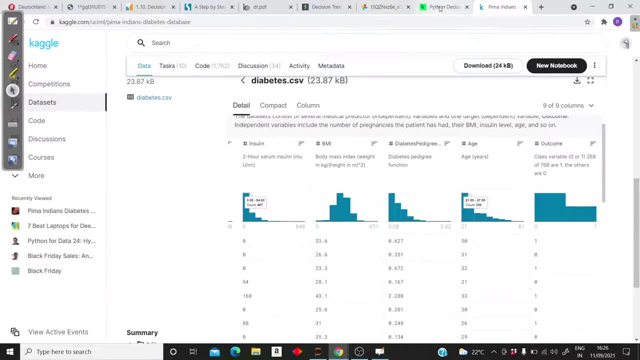 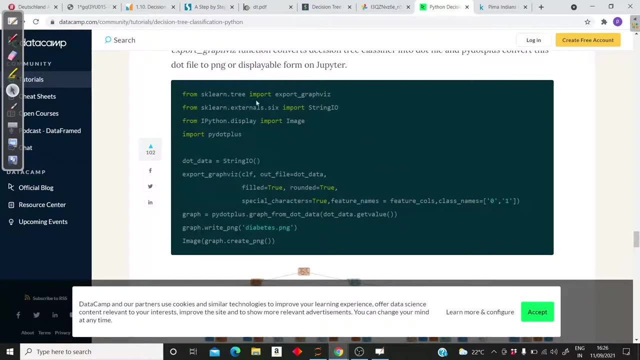 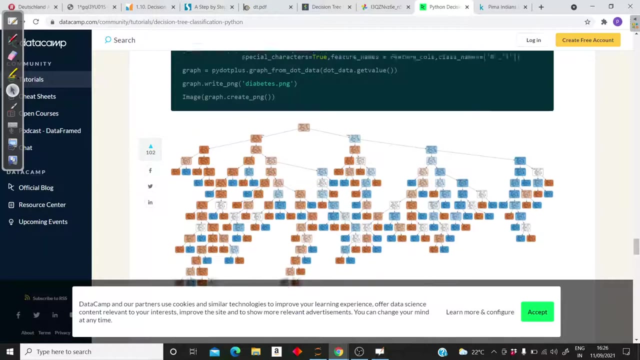 now how to visualize the tree, like as i showed you the tree so you can see here that. so you after, if you'll, so there is one code here that after having this entire tree built, you can just copy paste from here and then you will get this thing. i just opened it here so you can see that. 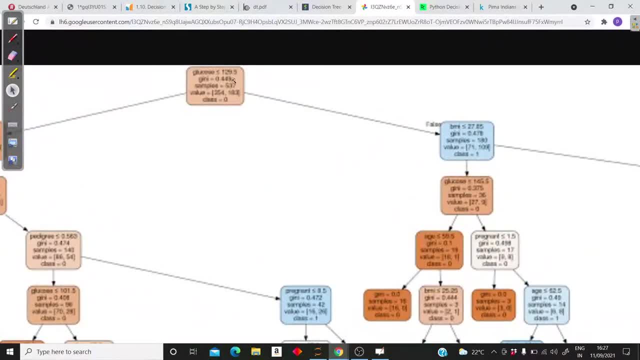 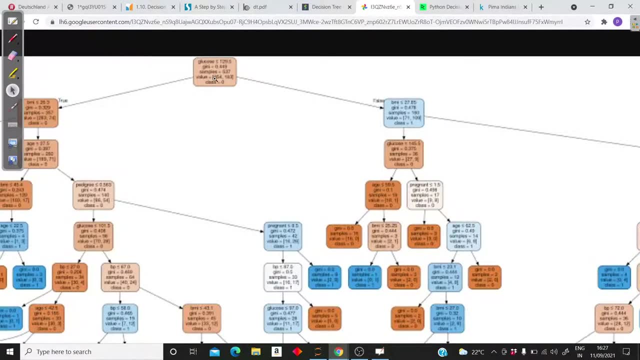 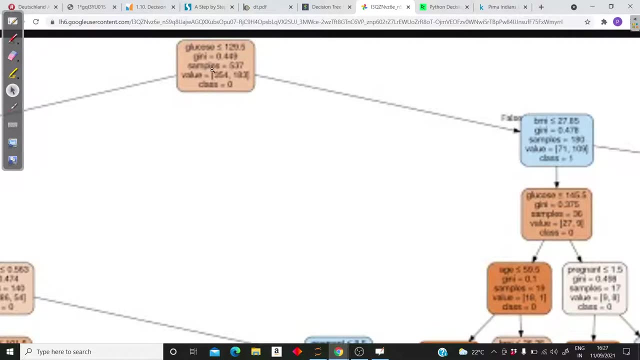 this is very hard to visualize like, because you can see they choose root node as glucose. i hope it's visible. it's little bit blur now, yeah, but i can interpret it. if you are watching in low quality you might not get it. so it's a glucose now and then there is some genie impurity, then samples. 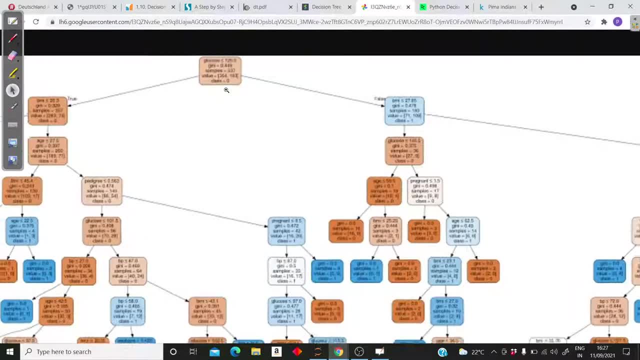 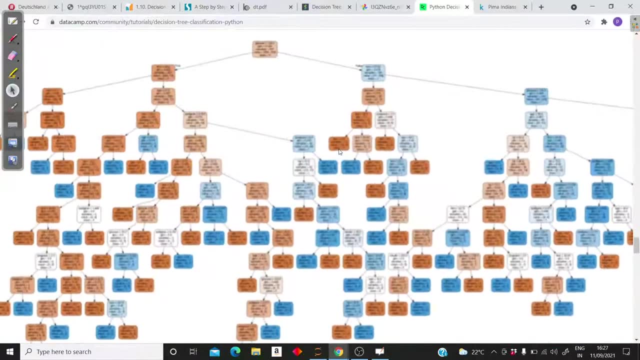 that how many are having glucose less than this value, and so on. so let's, let's go ahead and let's not not go inside. you can see from here- here as well, there is image like that, only so it. it won't be good to see. so this is like we are making the decision tree to the fullest. we are growing it to. 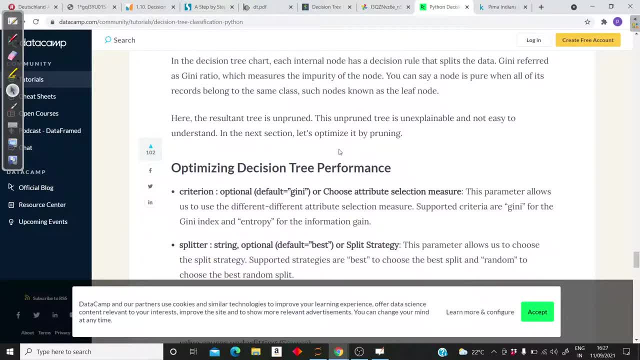 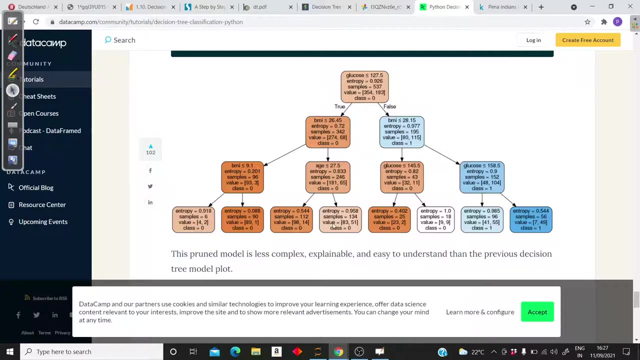 the fullest. but what we can do is that we can optimize it based on certain parameters. so if you will see the arguments of the decision tree, you can. you will find many things that we can optimize and after optimization what we'll get is this beautifully looking tree. so it's not like we 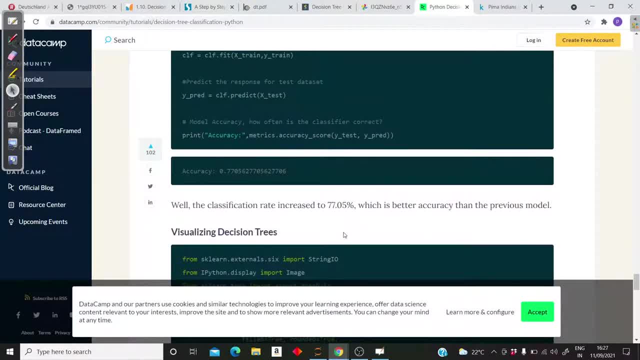 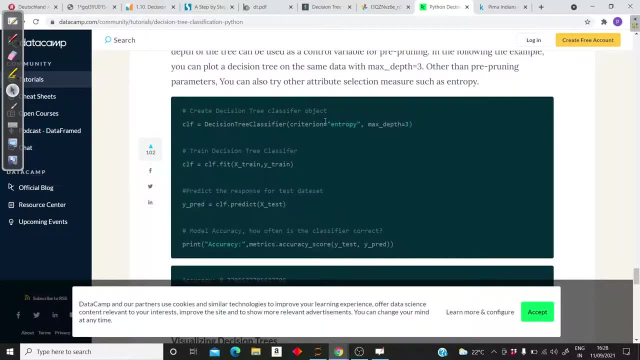 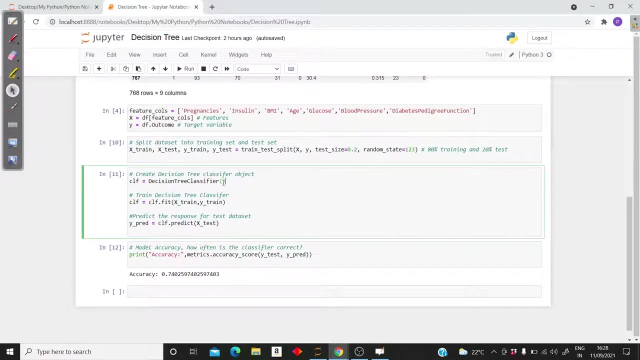 are going to the maximum depth, right, so i'll talk about this optimization. and even our accuracy can increase after optimization, so we'll talk about this optimization, like here you can see again we are so what we did here. let me just go there that here we just had decision tree and we didn't pass. 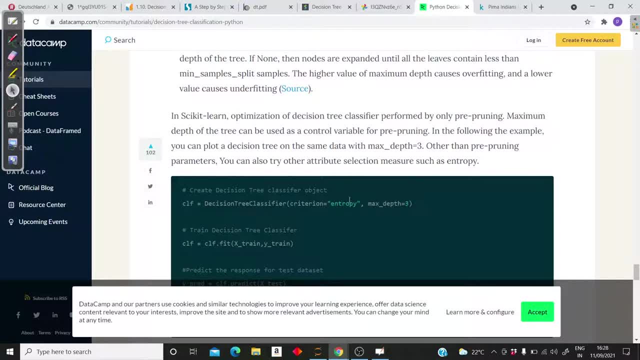 anything. so it took all the default values. but you can have criteria as entropy. we used genie like default. it is genie cyclist is using genie as a default criterion. so but here if you are using entropy you might get sometimes good accuracy, but in general both the methods are.